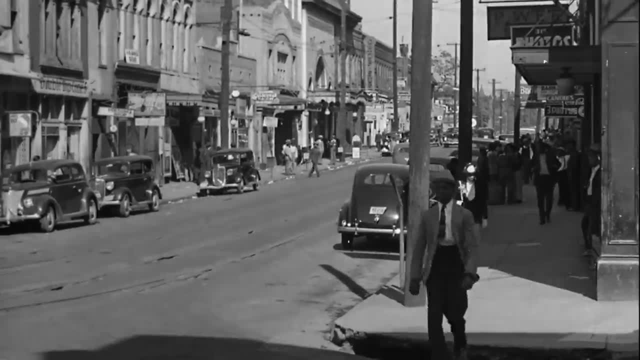 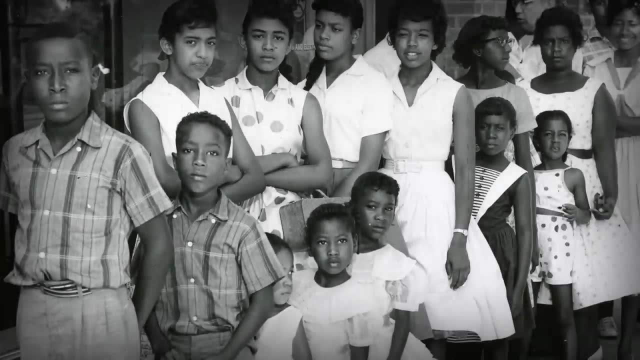 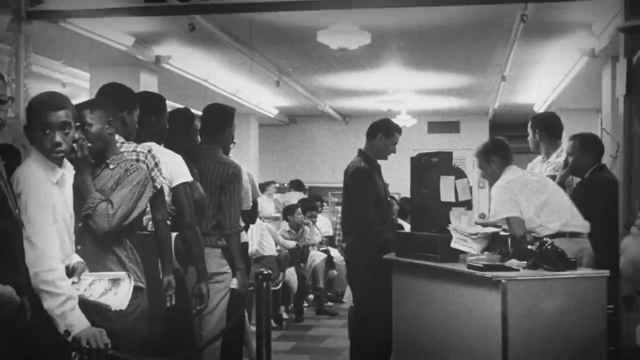 They knew the way their community was shaped, The way it was set up, was wrong. White people had more rights than African American people. The kids made a plan to fix things. But would it work? The kids decided to get the restaurants to change so that African American people were allowed to eat in them. 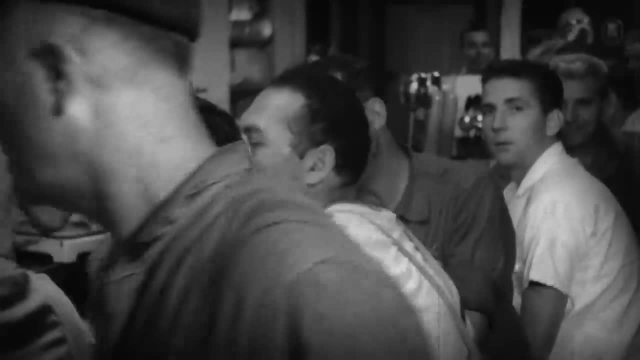 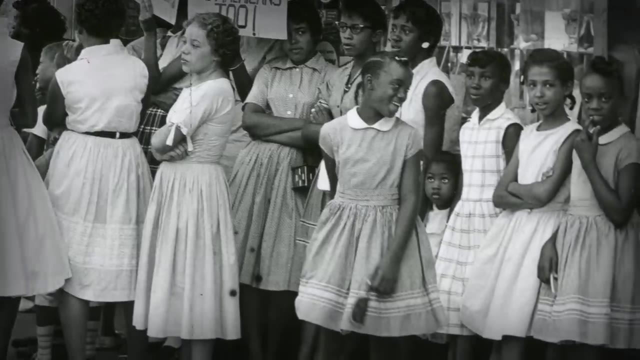 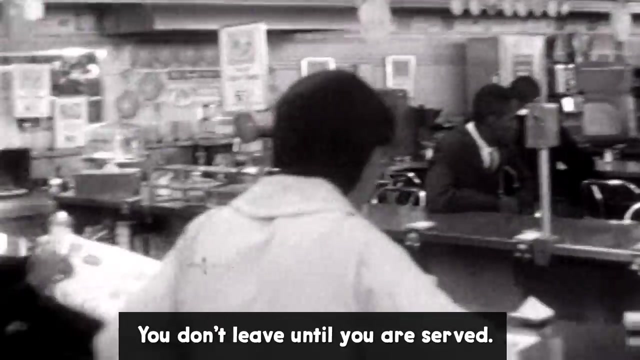 It could be dangerous to try to do that. Many people would be angry. but the kids were brave. They planned a sit-in. At a sit-in, you sit in a restaurant and ask to be served. You don't leave until you are served. 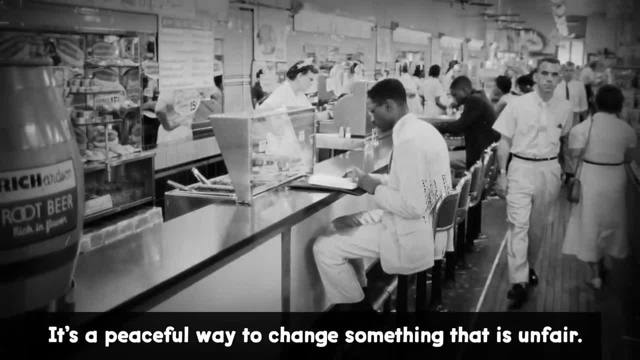 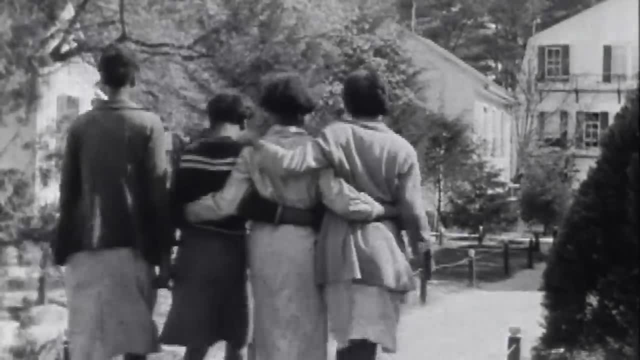 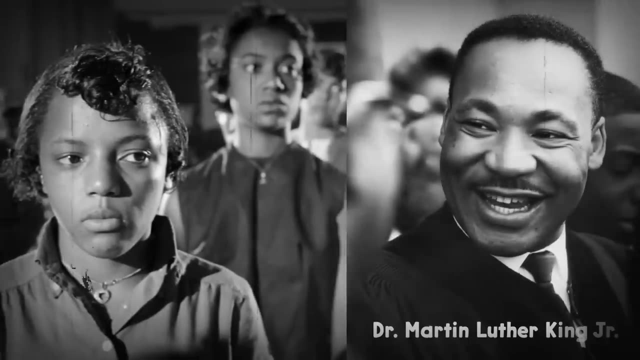 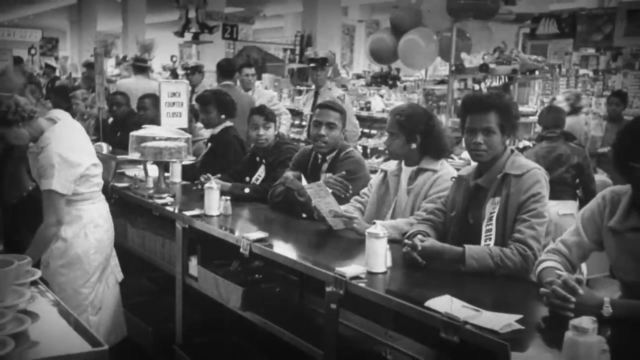 It's a peaceful way to change something that is unfair. The kids went into training with a group of African American adults. In training, these adults taught the kids about nonviolence. They taught them about Dr Martin Luther King Jr. Many people didn't want African American people to eat in a whites-only restaurant. 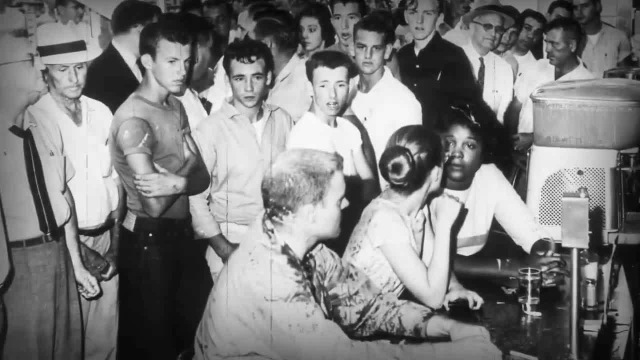 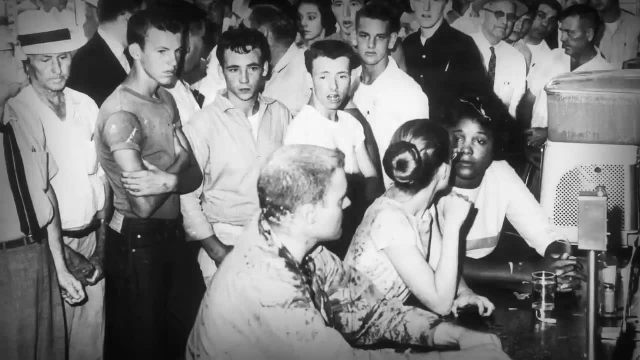 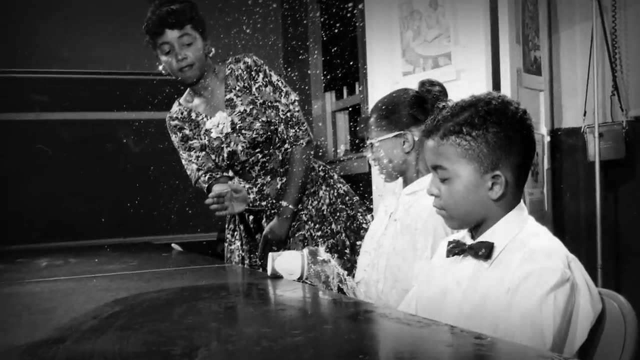 The kids learned that people would be unkind. The kids learned that they had to stay calm and be peaceful, no matter how badly others behaved. In training, the adults yelled at the kids. They threw water on them. The kids practiced being calm and not yelling back. 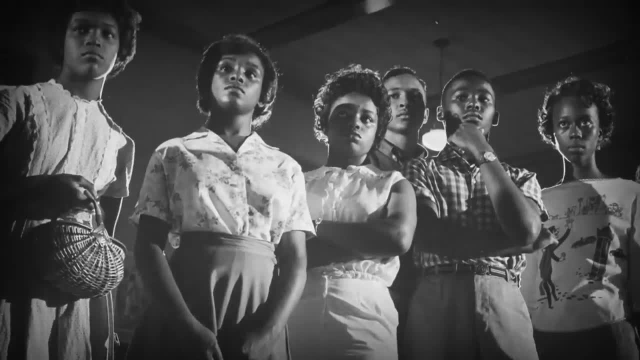 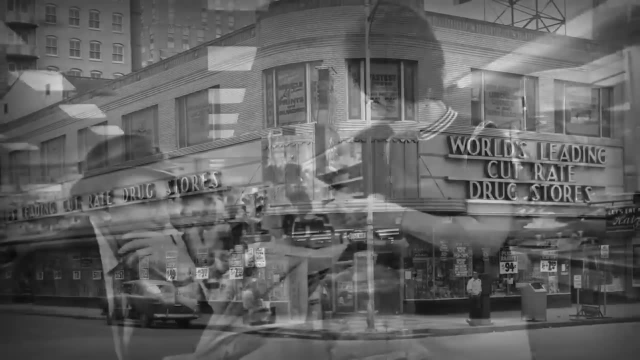 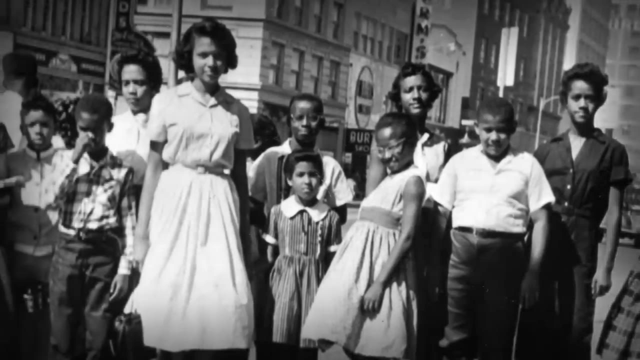 Soon they were ready to do their first sit-in. The kids' first sit-in was at the Cats' Lunch Counter. It was a whites-only restaurant. Ayana went with about 12 other kids. They all wore their best clothes. They went in and sat down. 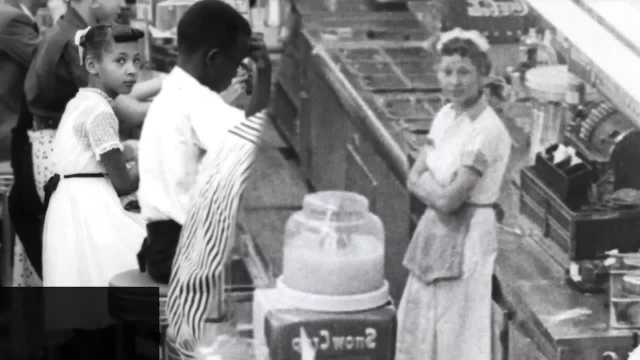 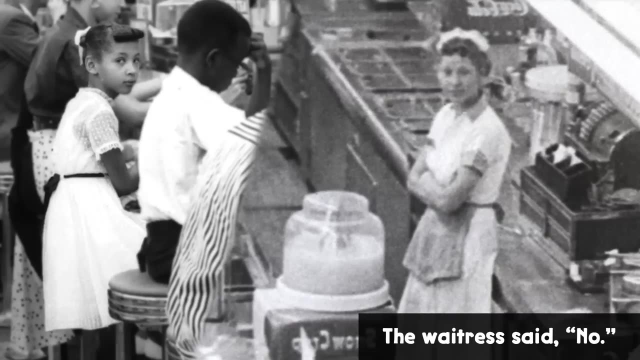 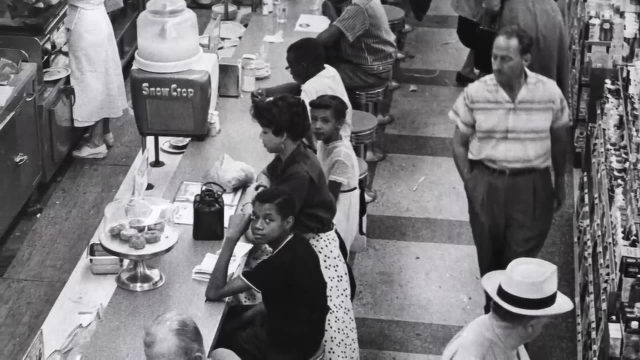 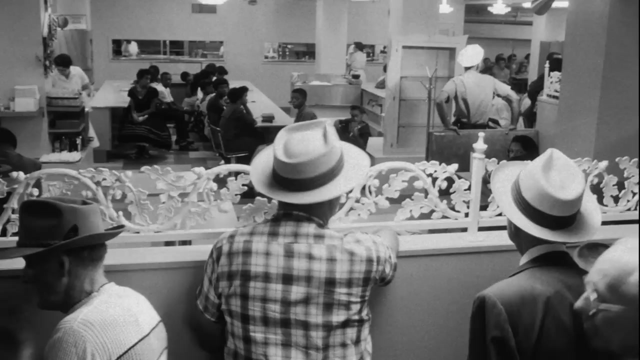 They were polite. Ayana asked for a hamburger. Ayana asked for a hamburger and a Coke. The waitress said no. The other customers were angry. They didn't like that. African American kids were trying to change the restaurant. They did not want it to be integrated so that everyone was allowed to eat there. 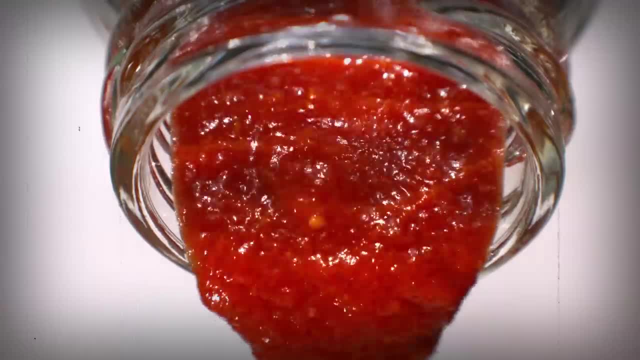 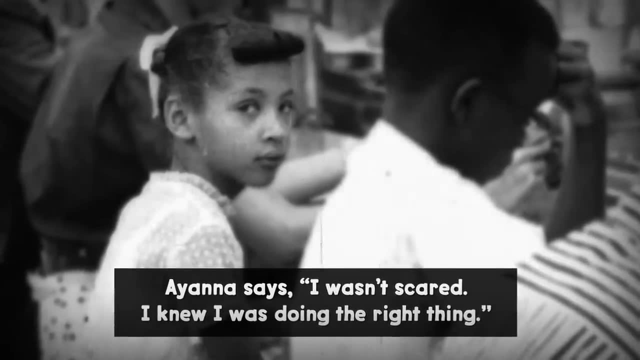 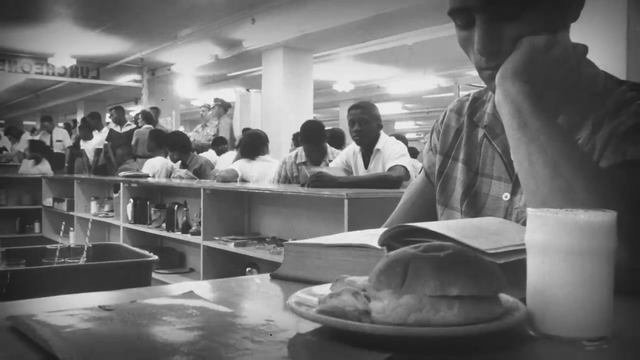 The other customers yelled at the kids. They poured ketchup and coffee on them. Ayana says I wasn't scared. I knew I was doing the right thing. The kids didn't yell, They didn't fight. They sat quietly and talked with each other. 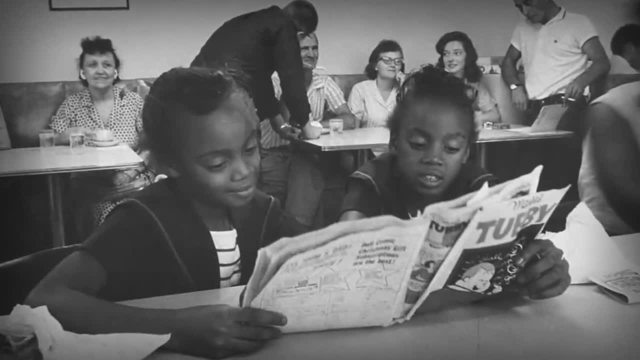 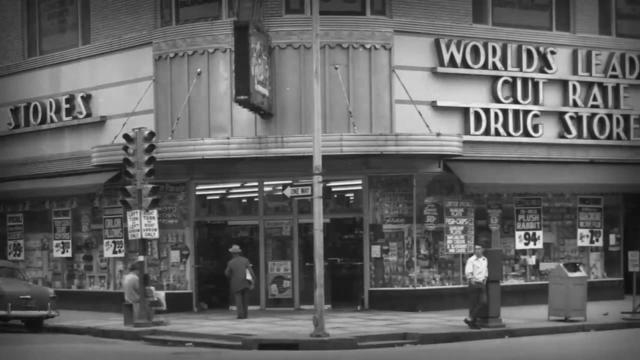 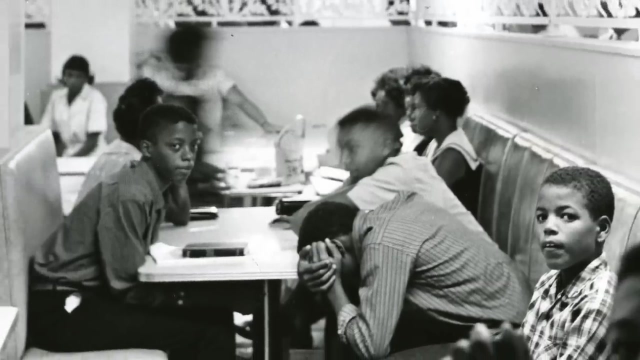 They had brought magazines and coloring books. At the end of the day the restaurant closed. The kids had to go. The next day they went back, They ordered food again. No one gave it to them, but they were not going to give up. 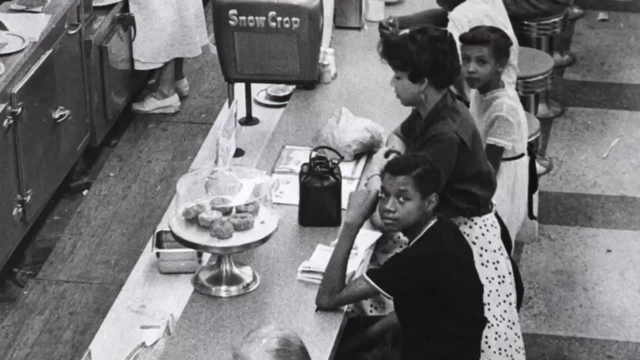 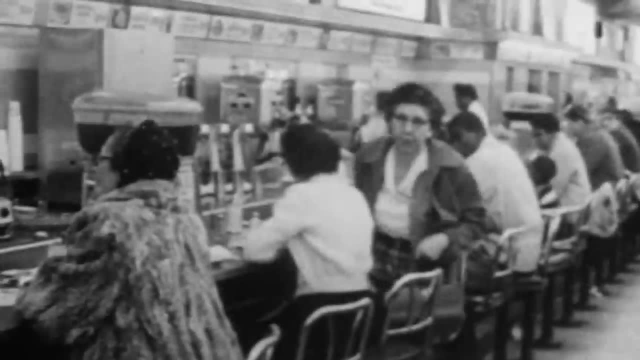 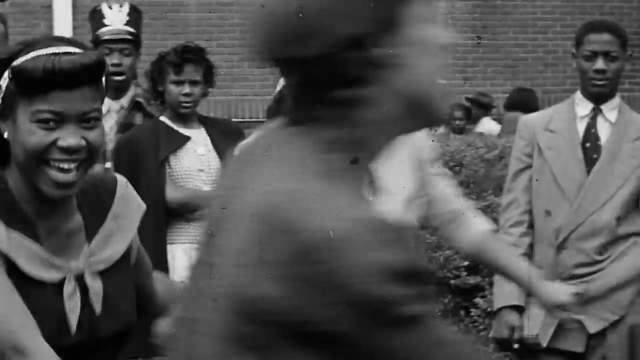 They were determined. On the third day the kids ordered food. This time the waitress brought it to them. From that day on the cat's lunch counter was integrated. Anyone could eat there. The kids were so happy They had made one place in their community better. 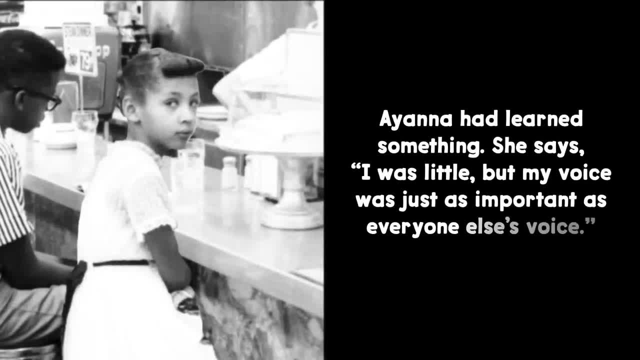 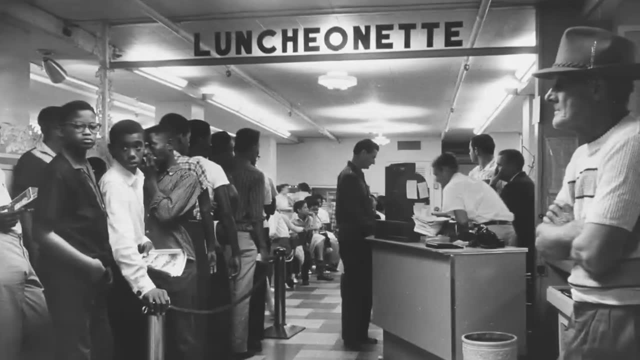 Ayana had learned something. She says: I was little but my voice was just as important as everyone else's voice. But their work wasn't done. So many restaurants in their community were segregated. Over the next six years the kids did sit-ins at many restaurants. 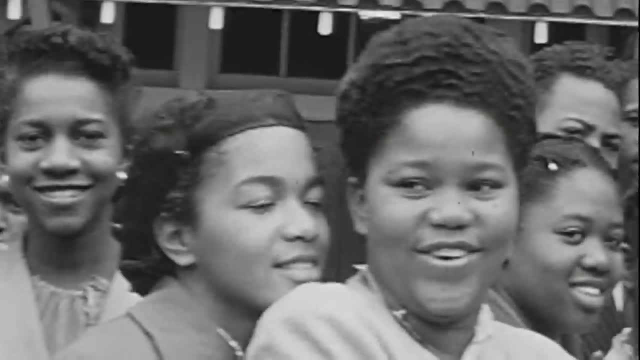 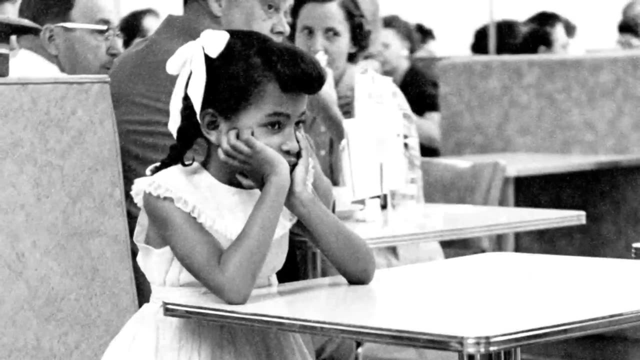 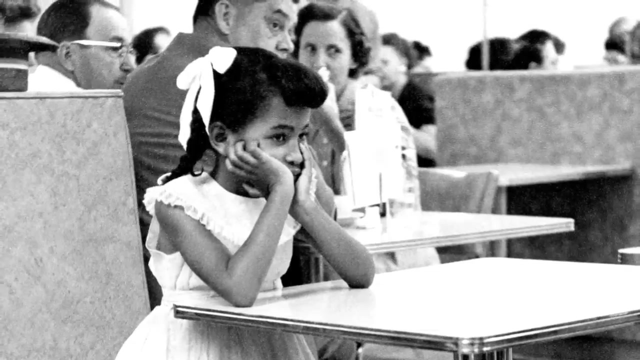 More and more kids joined. each time The restaurant owners got pretty clever about trying to keep the kids away. At one restaurant, workers took away all the chairs. There was no place to sit, But would that stop the kids? No, Ayana's little sister, Lana, had the right idea. 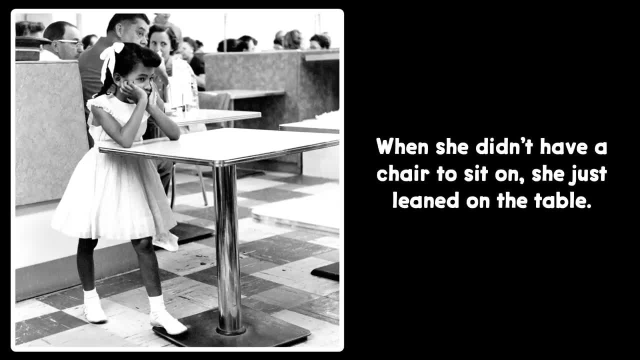 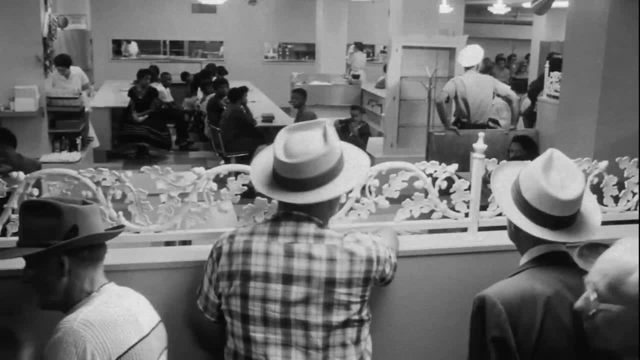 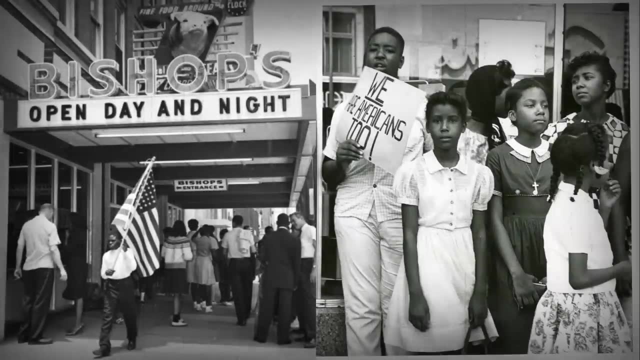 When she didn't have a chair to sit on, she just leaned on the table. In most places, people wouldn't let the kids use the bathroom. That wasn't going to stop the kids either. One by one, the kids integrated the restaurants in their town.